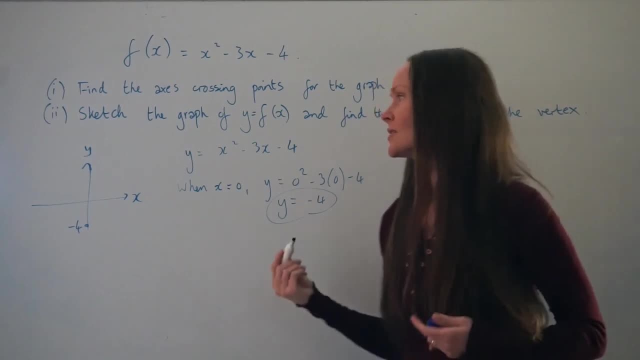 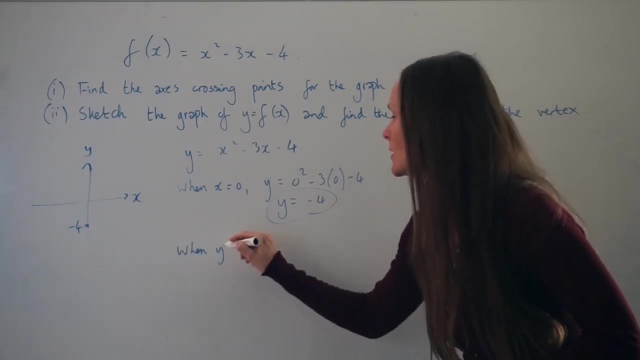 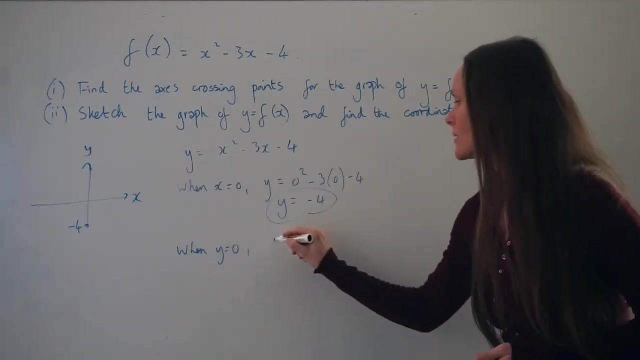 the x-axis. This time the y value changes to 0.. So that's always the case when a graph intersects the x-axis. So I'm going to change the y value to 0 this time, so that in this equation it becomes 0 equals. and then all of this, So in order to work out the x values. 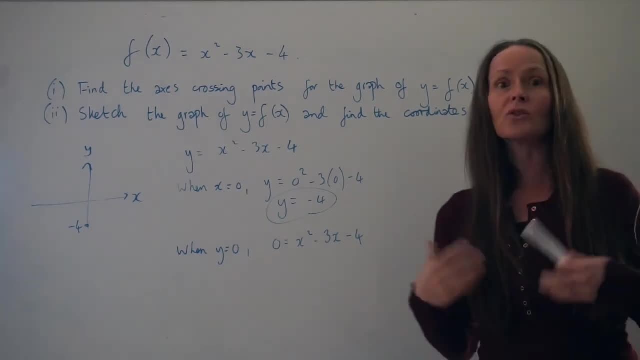 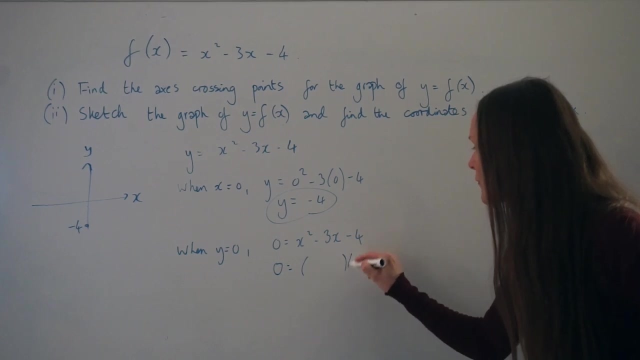 I have to solve this quadratic equation, So you could use the quadratic formula. or this one can actually work. So I'm going to use the quadratic formula, or this one can actually be factorized. So I'm going to factorize the quadratic and find the solutions that. 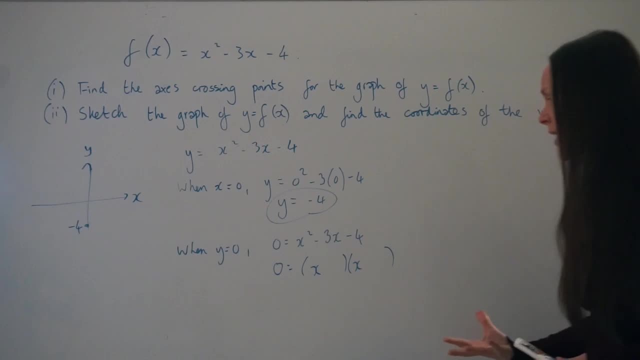 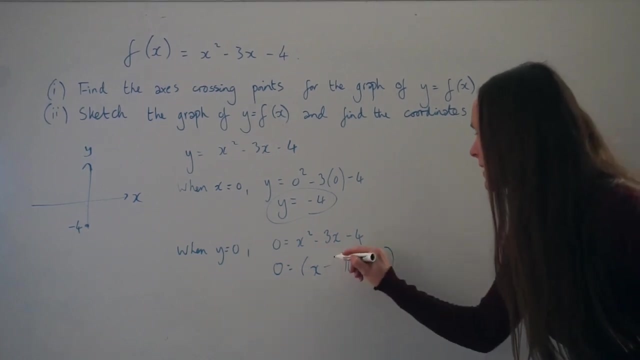 way. So remember, when you're factorizing you're putting into brackets these two numbers have to multiply to give negative 4 and add to give negative 3.. So they should be negative 4 and positive 1.. So my two x values are positive 4 and negative 1. So that means the quadratic. 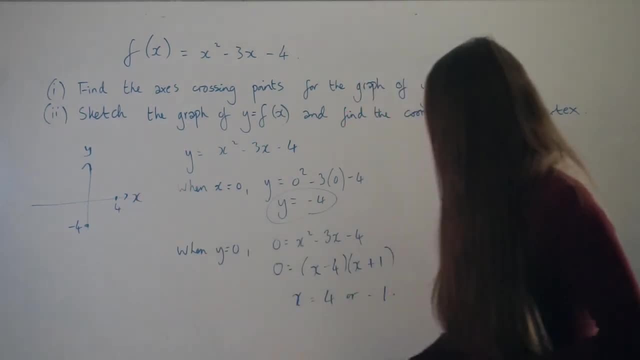 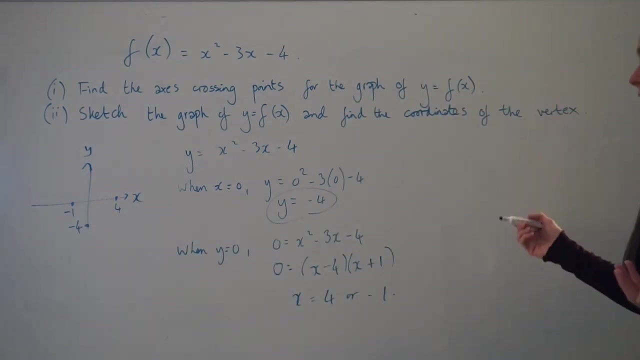 graph crosses at negative 4.. So I'm going to use the quadratic formula, or this one can be: a positive 4 and negative 1.. So when it says find the axes crossing points for the graph, y equals f of x, we've done it. I'm just going to write them as coordinates now. 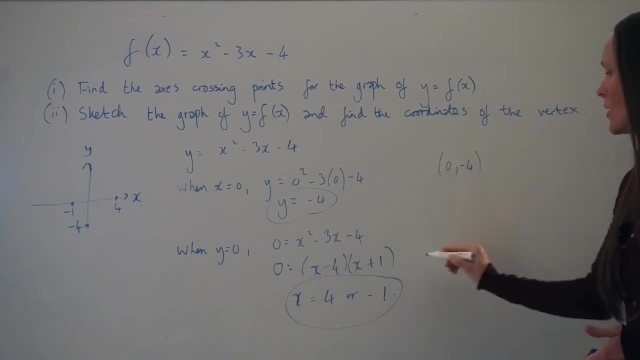 So we have this point here which is 0 minus 4, and then these two which are 4, 0, and minus 1, 0.. So there's part one. In part two it says: sketch the graph of y equals f of. 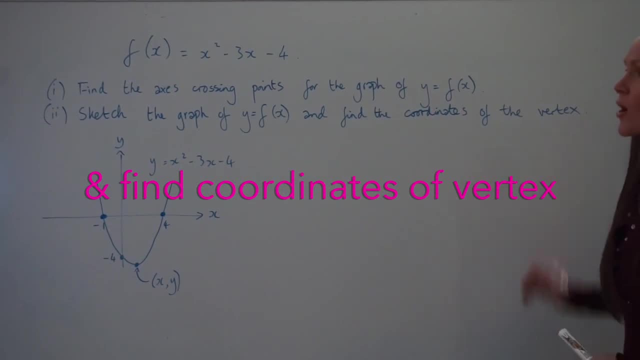 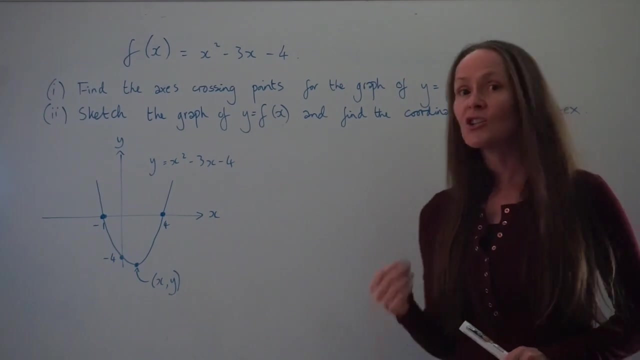 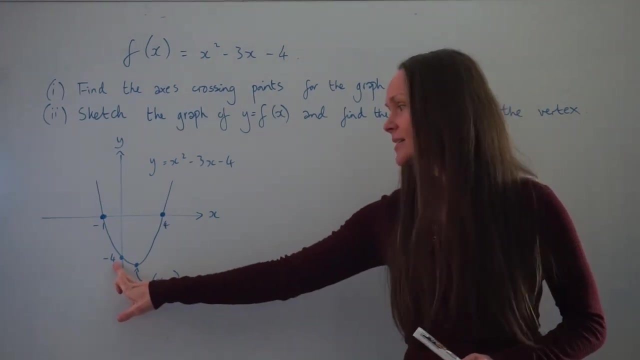 x and find the coordinates of the vertex. OK. so we have to do a sketch of the quadratic from earlier. I've just done a neater sketch over here showing the points of intersection that we just worked out. so where the graph intersects the x-axis and also where it intersects 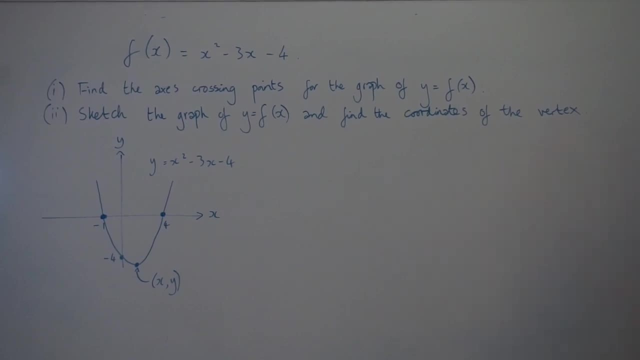 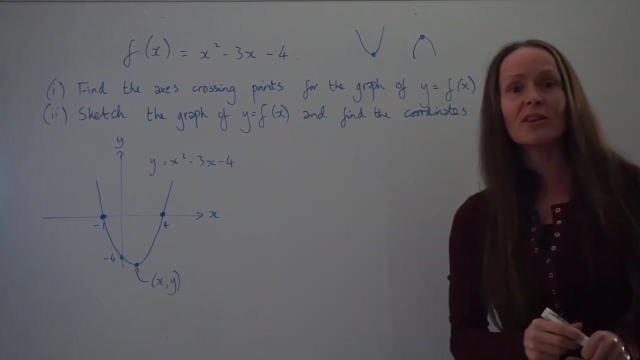 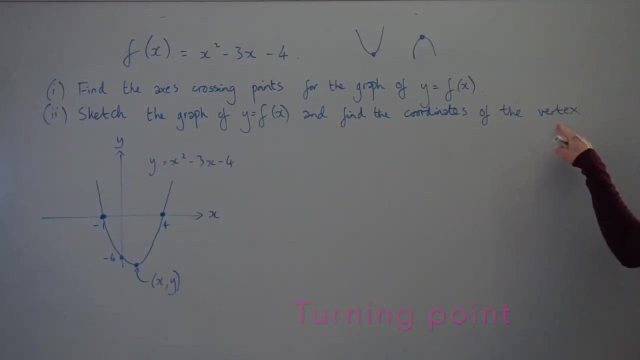 the y-axis. The vertex is either the minimum point on the graph or the maximum. Sometimes it might say find the coordinates of the stationary, Or it could say find the coordinates of the turning point. OK, they all mean the same thing as finding the vertex, All right. so something else I want to point out before. 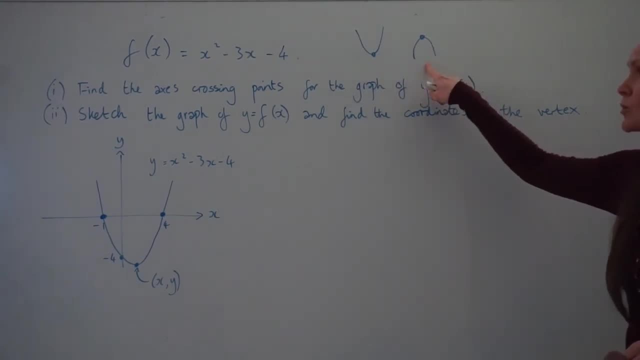 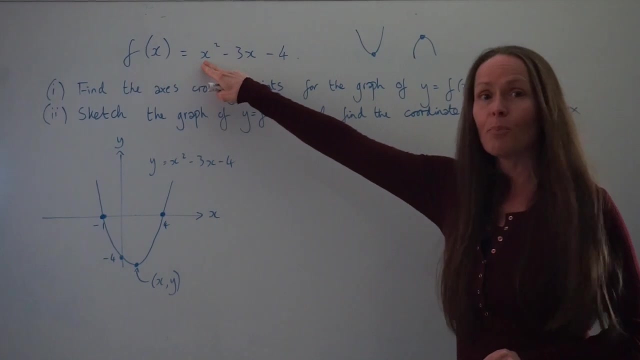 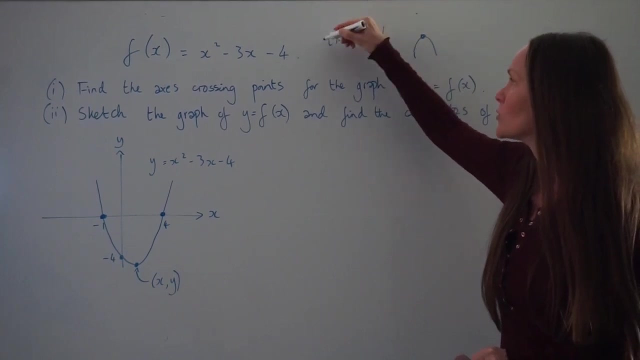 we try and work out the coordinates is which way you have to draw the quadratic. Is the parabola this way up or is it upside down, Whenever the x squared term here is positive? so if it's positive, x squared, like in this question, or 2x squared, or 12x squared, whenever, 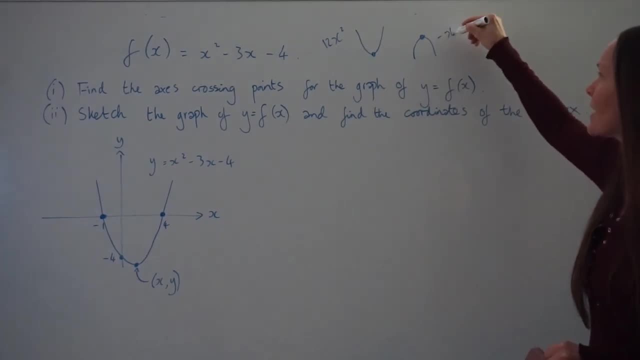 this is positive. it's positive x squared. So if it's positive x squared, like in this question, or 2x squared, this is positive. it's this way up. And whenever it's negative, so negative x squared, negative 3x squared, and so on, it's the other way. OK, so that's. 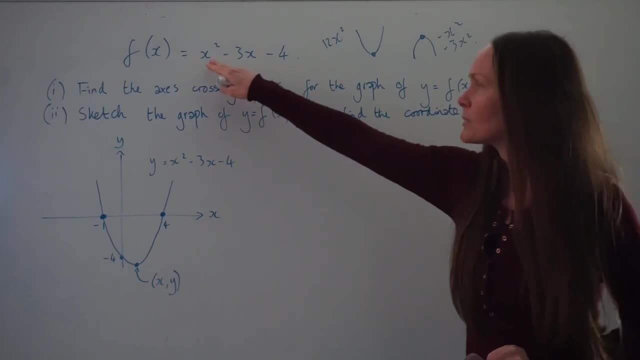 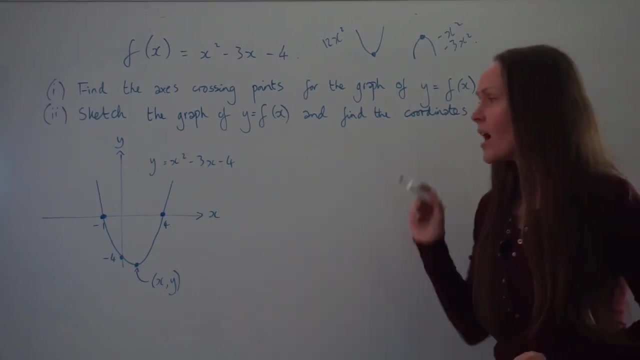 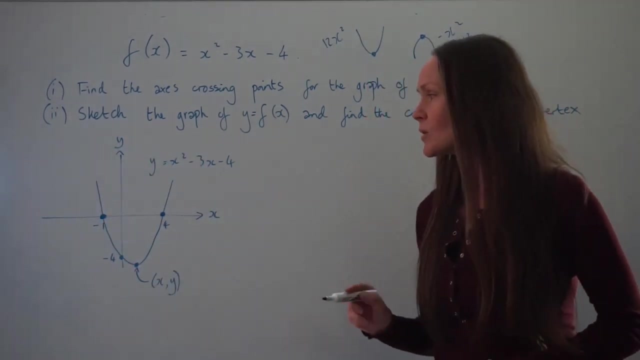 really important. So you can see, I've drawn it this way up because here it's positive x squared. So I'm going to show you two different methods to work out the coordinates of the vertex. Method one is to find the line of symmetry of this parabola, So the line of 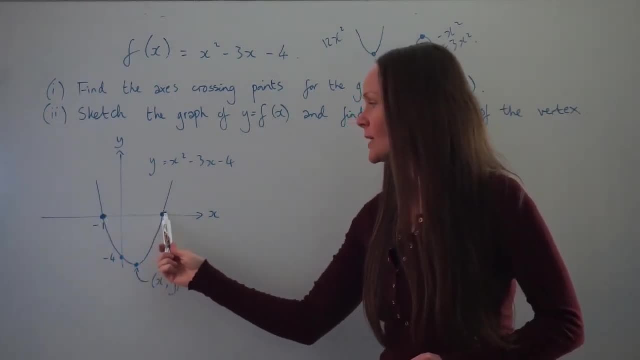 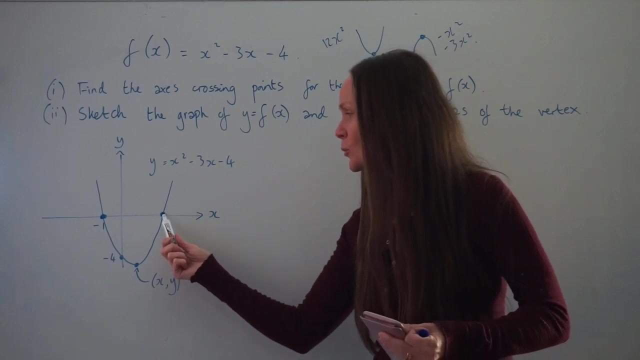 symmetry is always halfway between x and y, So I'm going to show you two different methods, these points of intersection on the x axis. So hopefully you can see there are five units between negative 1 and 4.. Half of 5 is 2.5. So if I subtract 2.5 from 4, it takes me to. 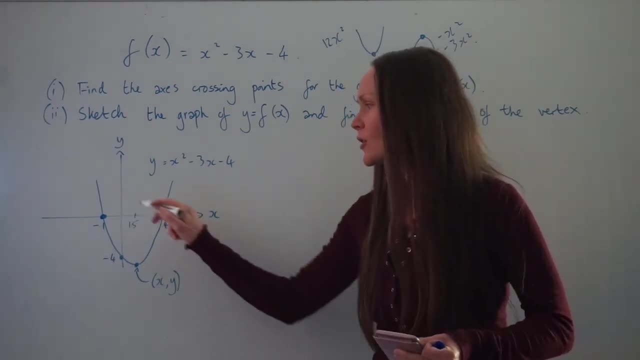 here, which is 1.5.. OK, it's just a rough sketch. I don't have to mark all the numbers on this graph. I'm just going to mark 1.5 and it's halfway between there. So this is. 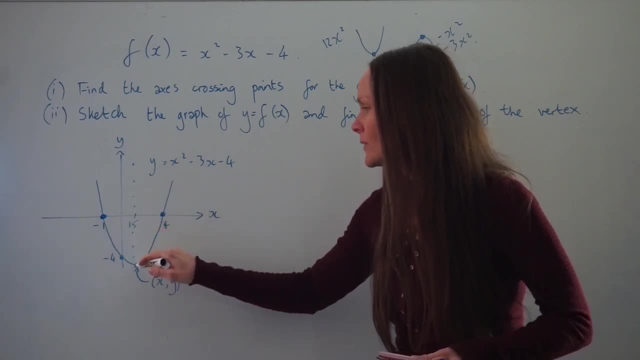 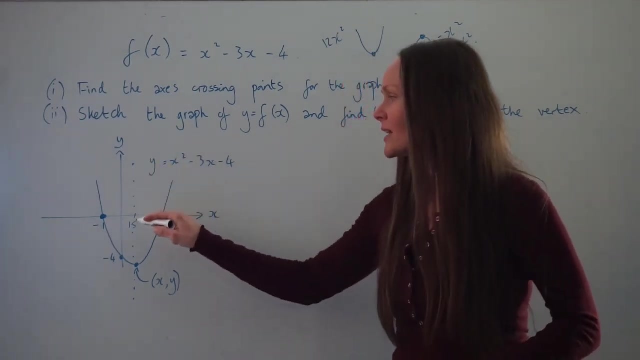 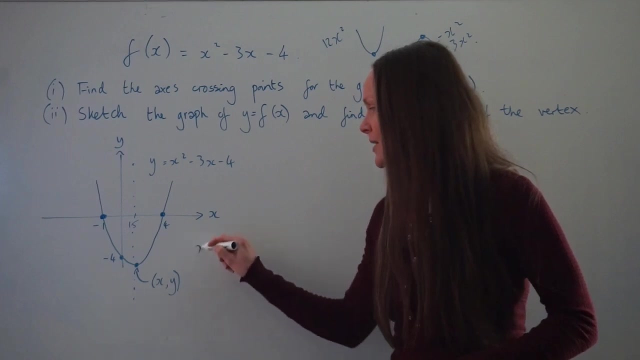 the line of symmetry of the parabola And the vertex point falls on that line of symmetry. So if this is the line, x equals 1.5, we've already worked out the x value of our vertex. The x value has to equal 1.5. 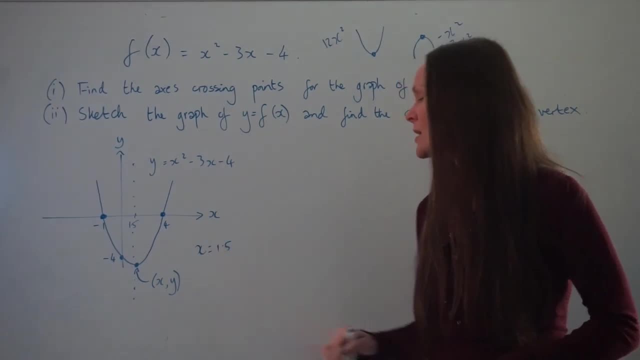 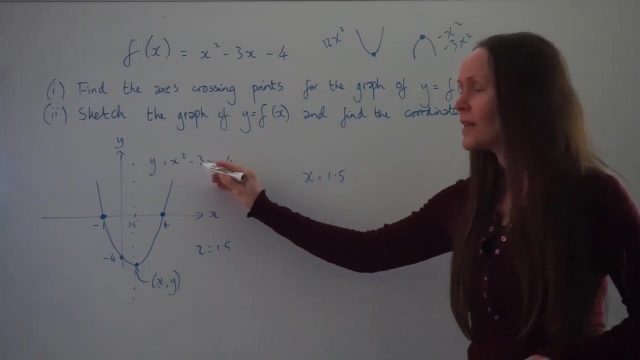 because it lies on the line of symmetry. OK, so x is 1.5.. We've already found part of it. OK, this part here. To work out the y value that corresponds to this x value, all you've got to do is substitute this number into the equation here. So to work out y, you change. 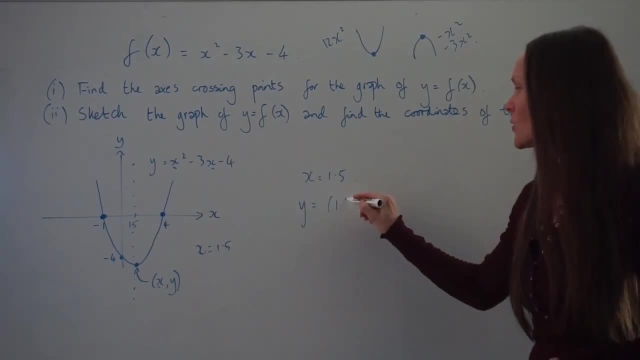 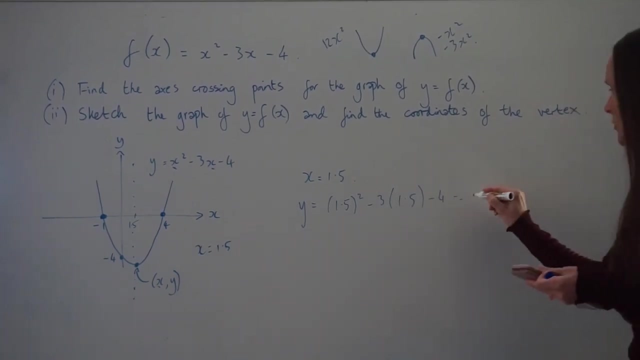 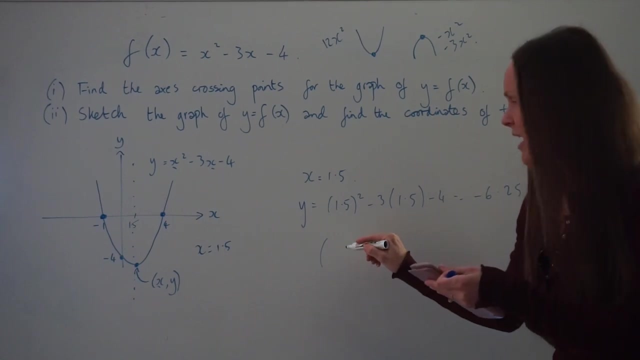 this x and also this x to 1.5, so that you have 1.5 squared minus 3, lots of 1.5 minus 4.. And when you do that you get negative 6.25.. So there's the value of y, So the vertex. 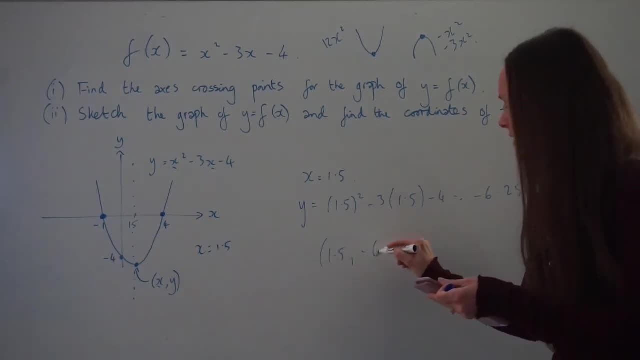 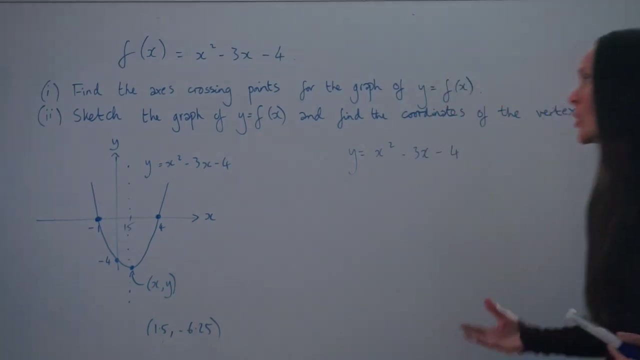 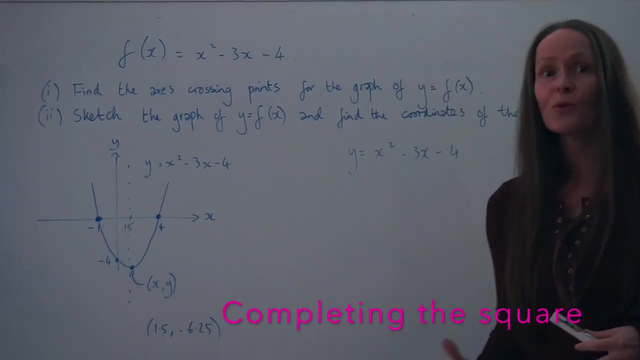 has coordinates 1.5, negative 6.25.. So there is method one. Just to finish, I'd like to show you an alternative method for finding the coordinates of the vertex, And this method is called completing the square. Now, if you haven't heard of completing the square before, I do have another lesson on. 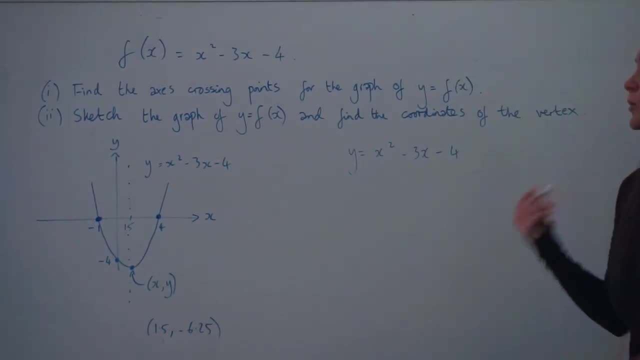 that if you'd like to watch to get some extra practice. So what you need to do first is start by writing out the equation again of the function, And this time we're going to complete the square. So rewrite the right-hand side of this equation. 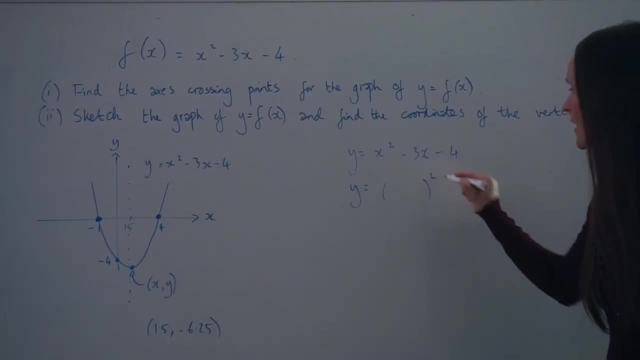 In completed square form. So to do that you need to have square brackets. First I'm going to fill in the x value. This number here is always half of the coefficient of x. So half of negative 3 is negative 1.5.. Or you can write it as a fraction if you prefer. Then 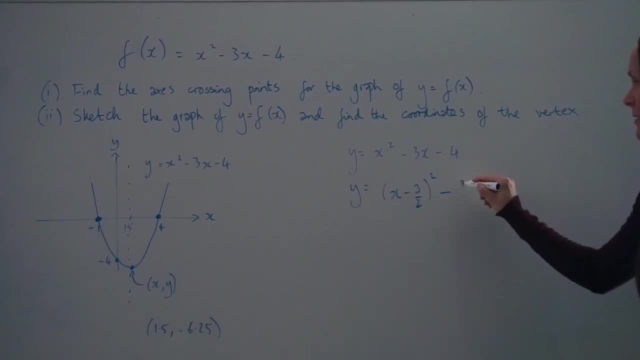 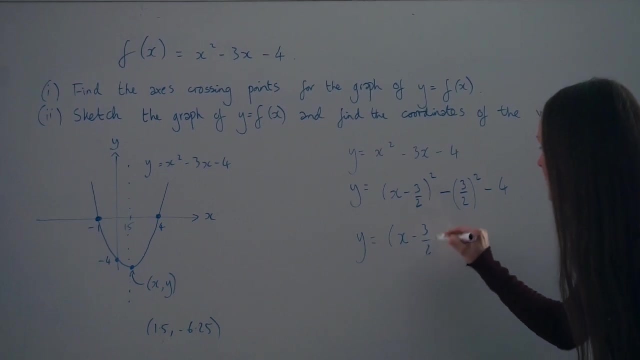 you have to subtract this number squared And then you would minus 4.. So this is just the method to rewrite in completed square form. Now I'm just going to calculate this part, So when I do that, the equation will now be: 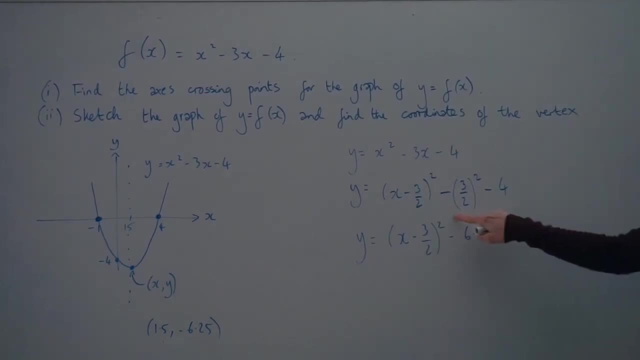 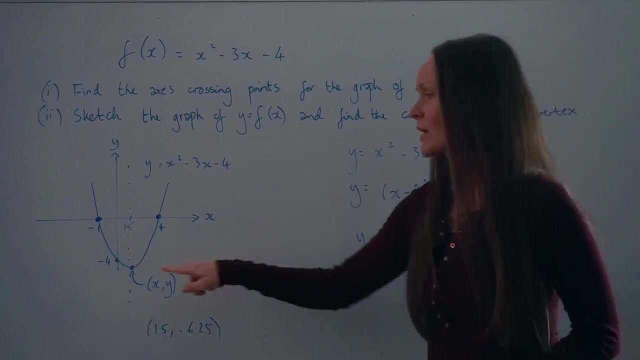 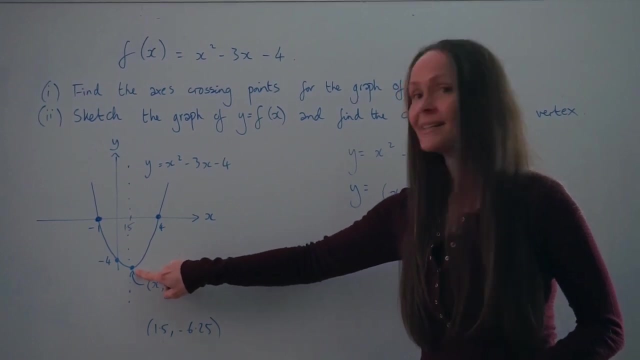 written like: so. So it's negative 6.25, if you work this out, which maybe you recognize from earlier. Now, if we look at the graph in this question, the vertex is here And it's the minimum point on our graph. So that just means y is at its smallest at the vertex. 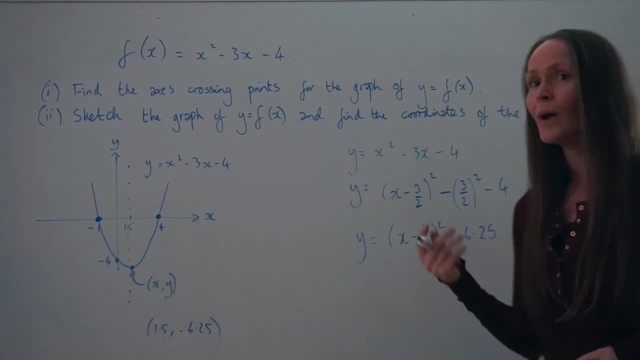 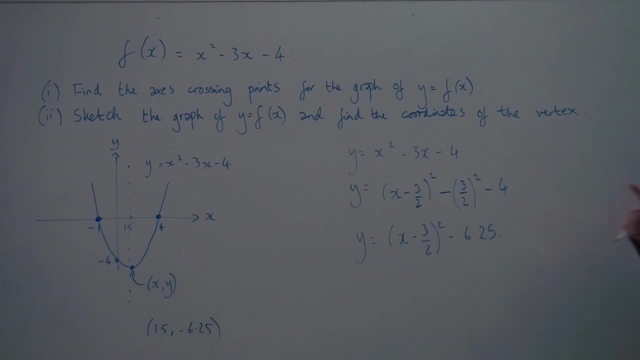 on this graph. Okay, So when y is at its smallest. So just bear that in mind. If we look back at the equation here, y is at its smallest, at negative 6.25.. And I'll just explain why. If you consider: 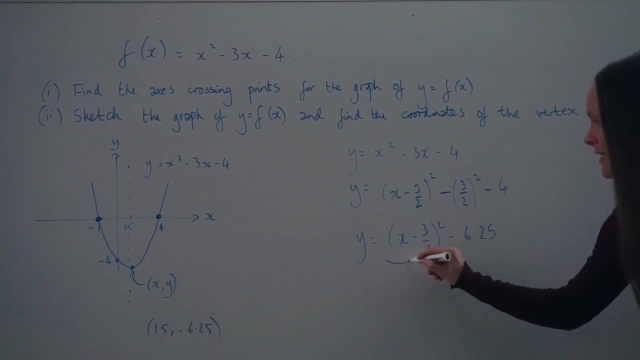 square brackets. the smallest square brackets can ever be is always going to be 0. This can never be a negative number, Because if you have a negative number inside the brackets when y is at its smallest, it's going to be 0.. 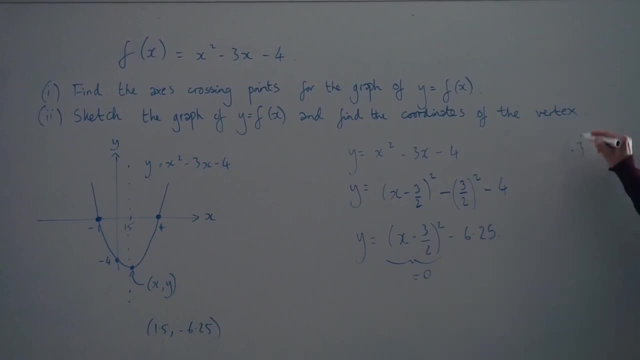 When you square it, it would give you a positive number. If you have negative 3 squared, negative 3 multiplied by negative 3 is 9.. So this can never be a negative number. The smallest it can be is always going to be 0. So if this is equal to 0, it's going to disappear And